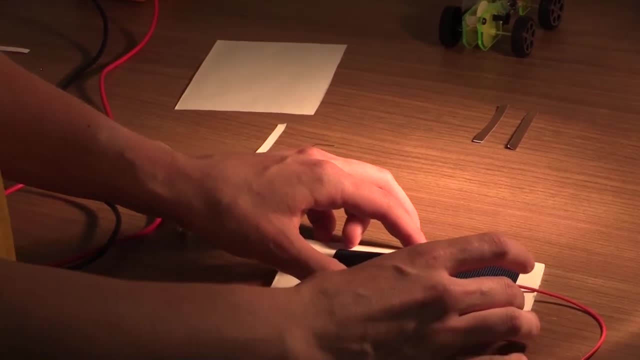 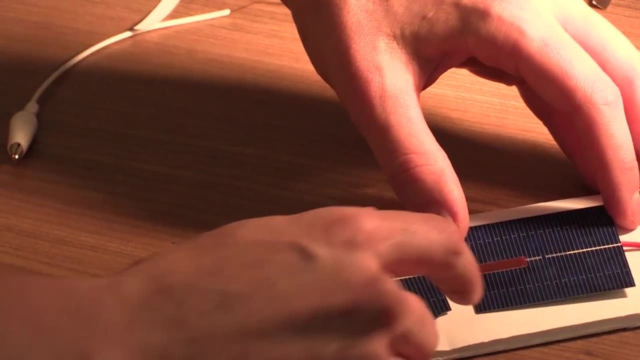 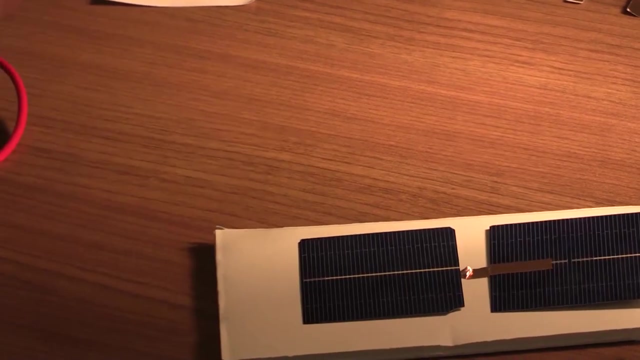 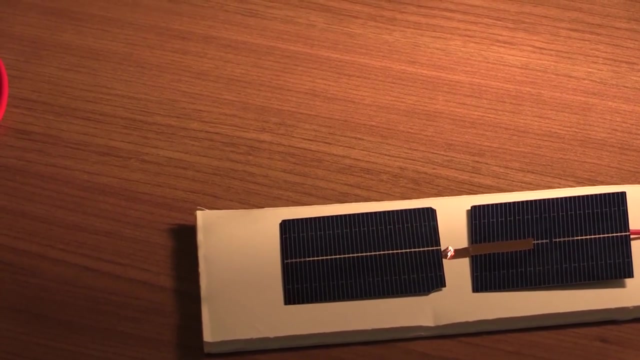 solar panel And we want to make sure that the copper tape doesn't end up sticking to the front side of this or the back side of our first solar panel. Now that we have a wire, our panels connected, we can go ahead and attach our last wire and test our device. So I'm going to peel off the copper tape again. 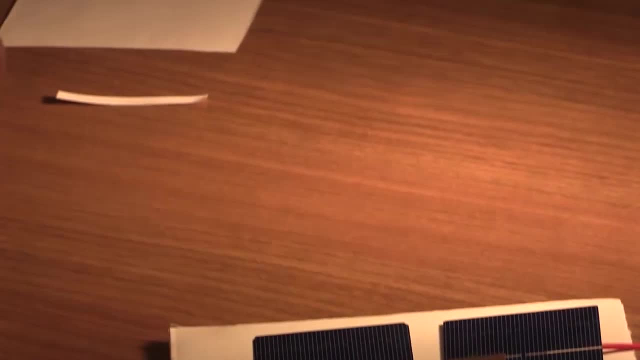 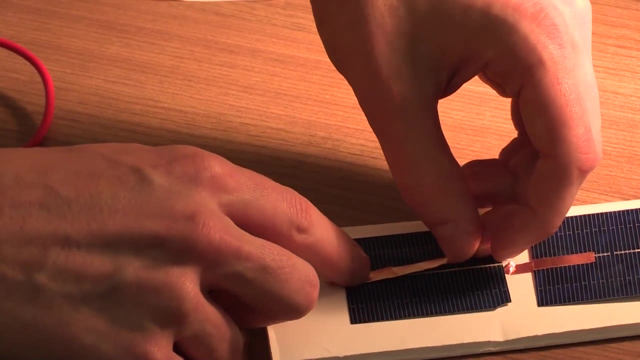 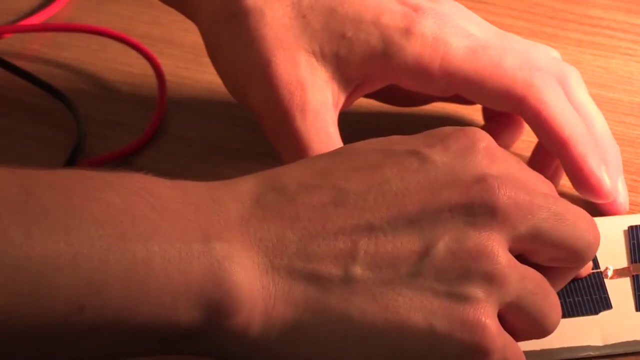 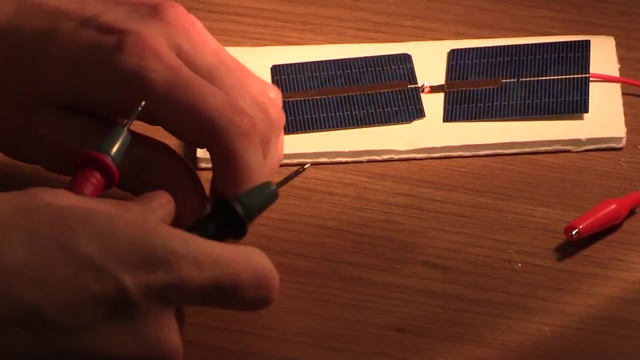 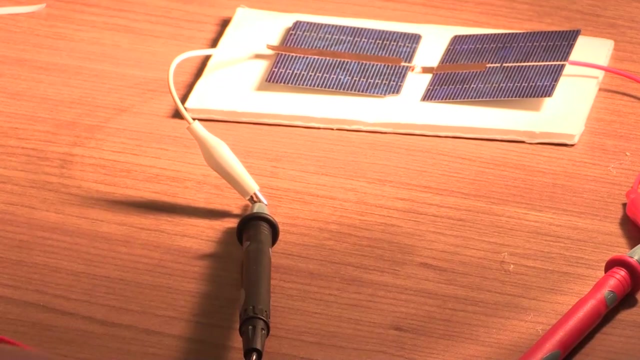 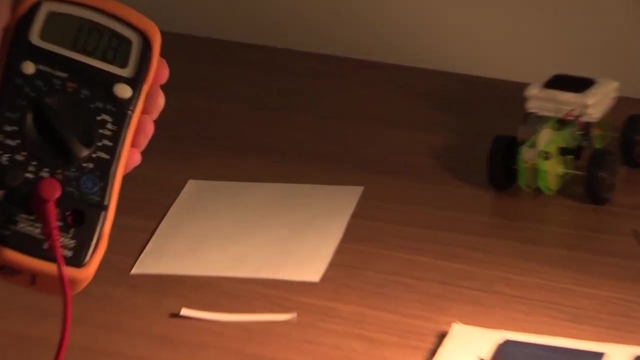 attach it to the exposed copper wire on the clip lead and then place that over the white contact on this solar cell. Now I have two solar cells attached in series and I can go ahead and attach them to my voltmeter. So when I measure the voltage I read about 1.8 volts. 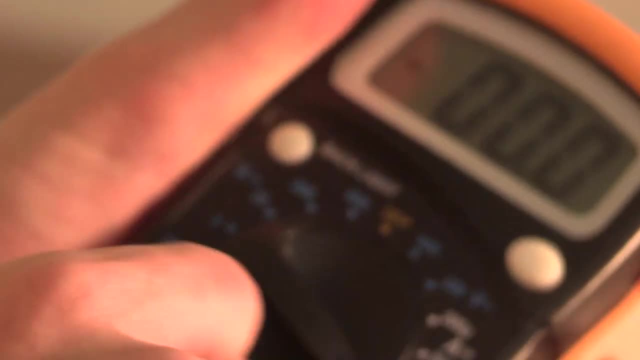 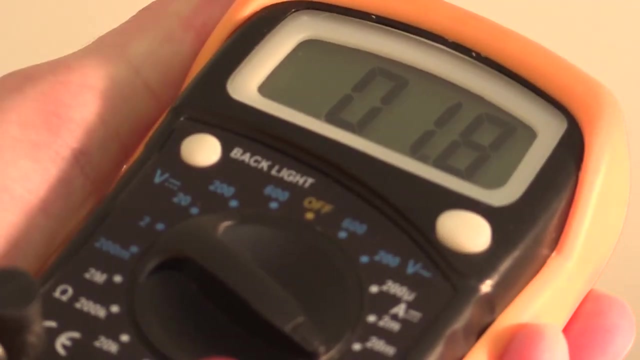 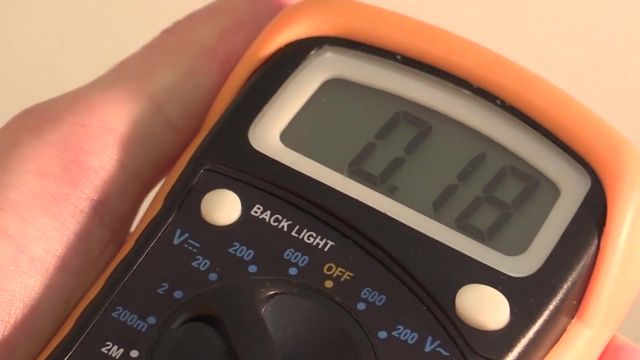 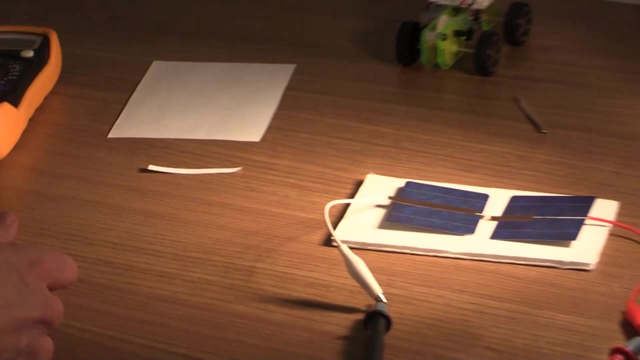 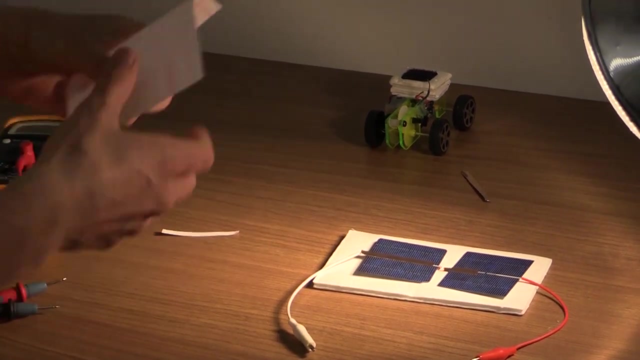 And then I'm going to switch over the lead and I can read about 180 milliamps of current on my solar cell. If I multiply those two together, that would give me the power of my solar cell. But for the last step that I'm going to do is I'm going to protect my solar panel by 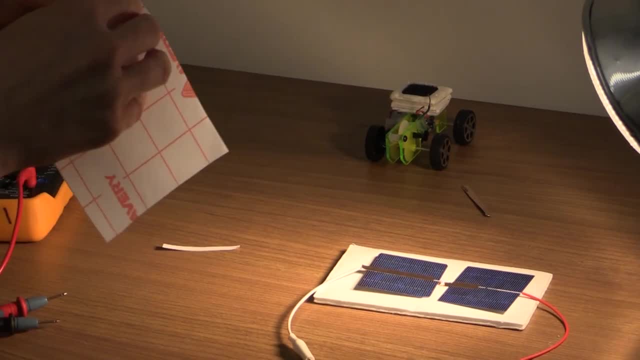 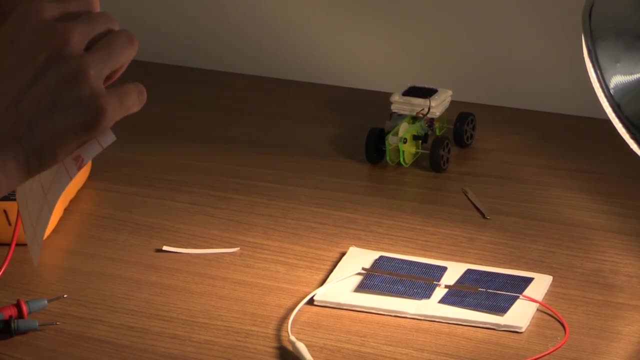 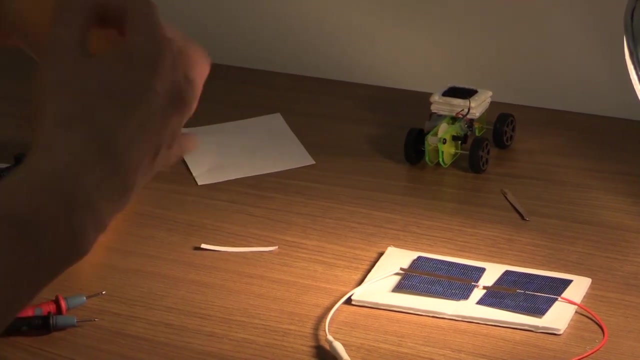 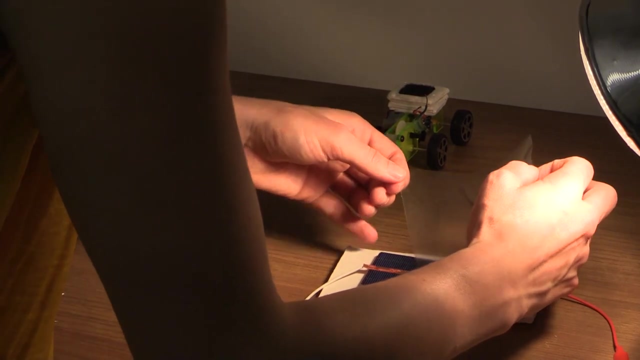 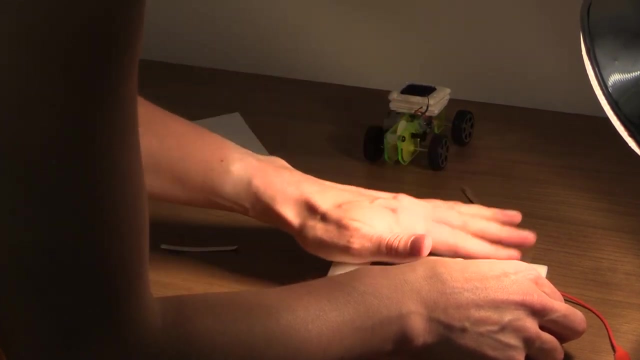 putting on a laminating cover over the panels, And this will help keep them attached to the foam board so that they won't get broken as easily. And so, for this, I just want to make sure that the cells are placed in the right position, and now I'm going to place the laminating tape over them.